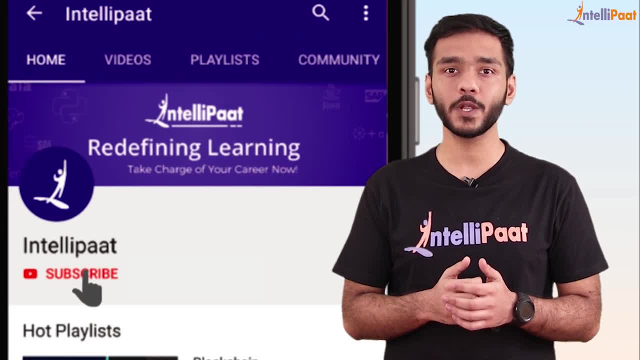 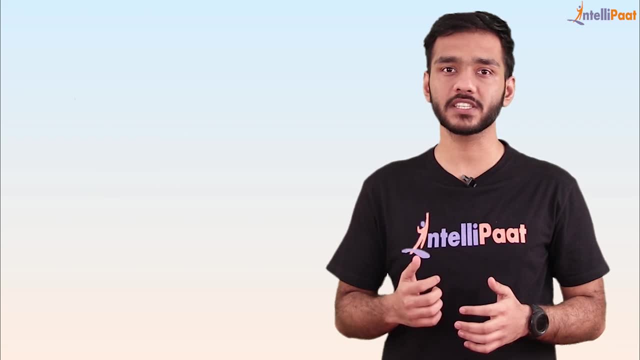 comes in our topic for the day. Okay, guys, before we get into it, make sure that you subscribe and hit the bell icon so you don't miss any of our future updates. Okay, guys, now let's take a quick look at our agenda. First, we will discuss what the 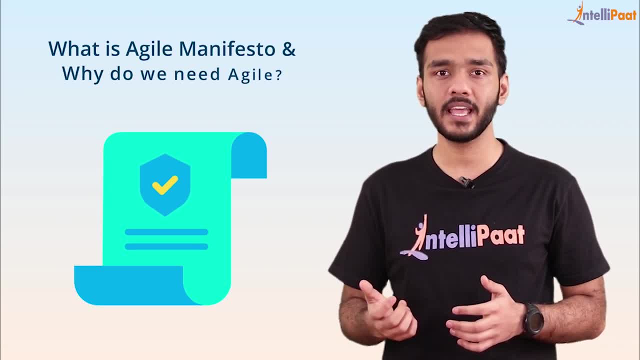 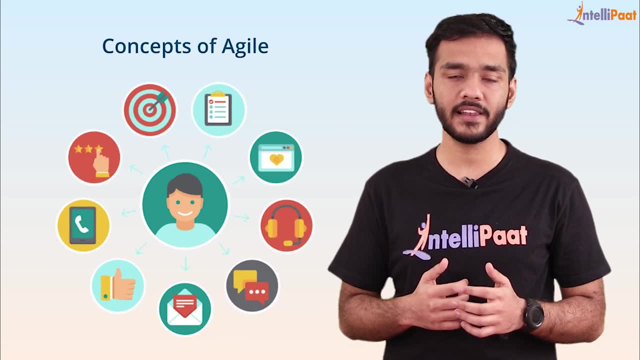 Agile manifesto is and why do we need to use Agile in the first place? And then we will learn what exactly Agile is, After which we will talk about the different concepts of Agile, and finally, we will conclude by discussing how we can implement Agile ourselves. 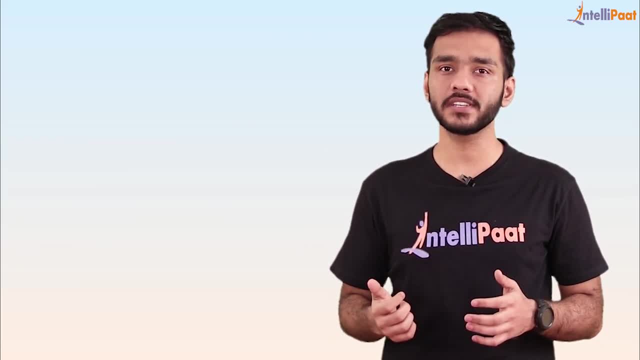 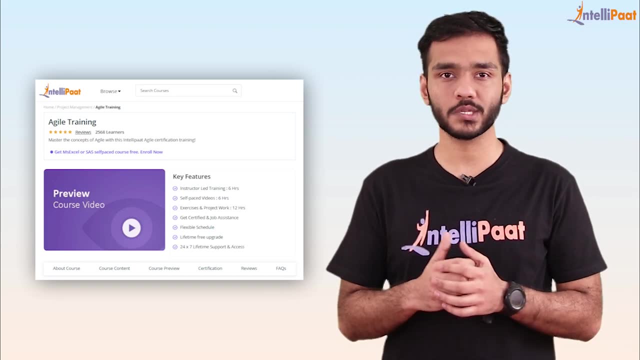 and how does it actually work? Also, guys, if you're looking for end-to-end training in Agile, we do provide the same. For any further details, please check out the links given in the description below. Now let's start the session. 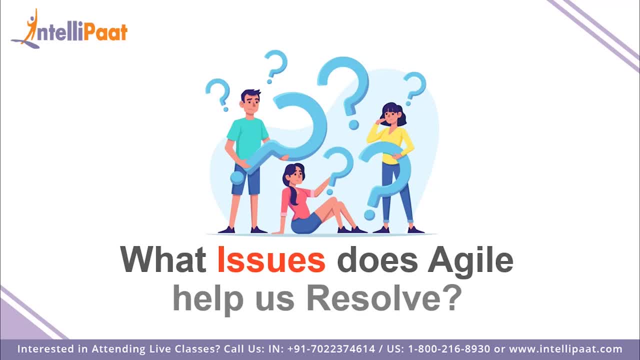 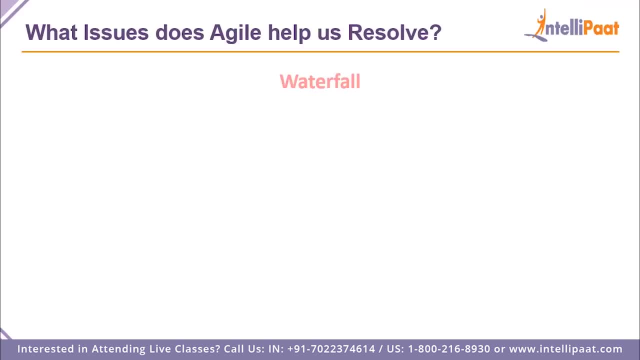 Let's start off by discussing what issues does Agile have to deal with Now? to discuss this first, we have to go and look at the previous methodology that was used. Now, traditionally, waterfall model is the one that was used for software development. 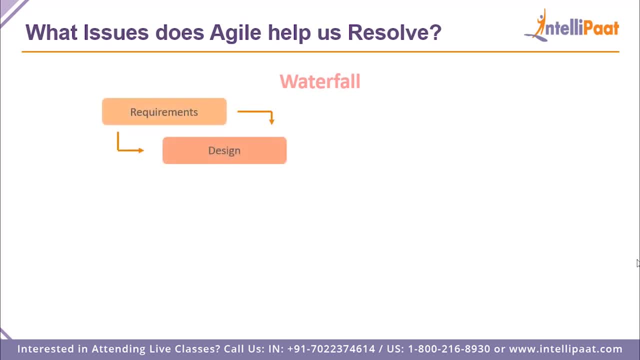 Now the waterfall model consists of various phases. You have your requirements phase, your design phase, implementation phase, testing phase, deployment phase and maintenance phase. Now waterfall model as a whole promotes a very long-term development lifecycle and it was used to develop monolithic applications. instead of the microservices, we have these. 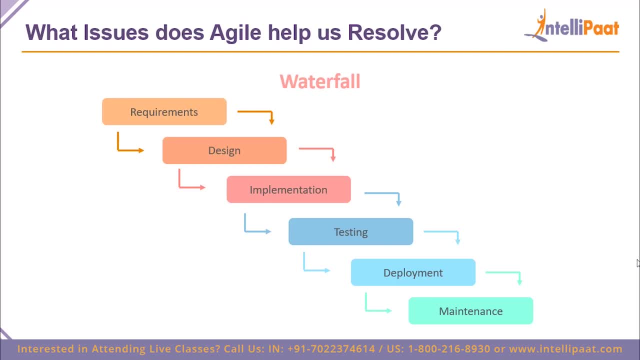 days. So now we can see how these issues start to develop. As you can see, with waterfall you need a very long time to develop a particular software. These days this is not feasible, as the demand for software is crazy high and we need to be able to change according. 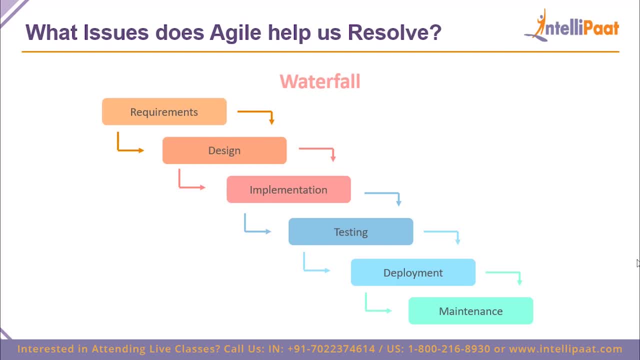 to the market's needs and, you know, develop software every other month or so And because of these issues, a new, particular software methodology was created to tackle the issues, And this is where Agile comes in. So with Agile, you're not creating software in a very long. 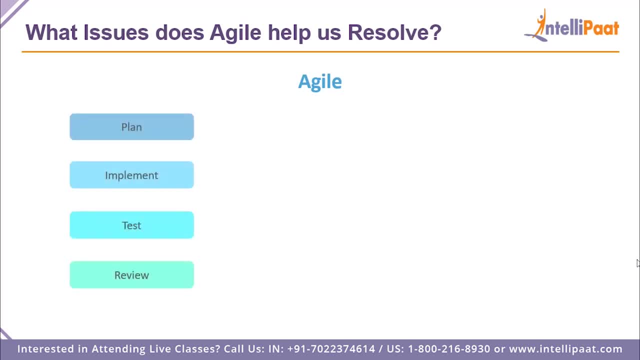 period, whereas you'll be doing it in multiple sprints. You will start off with the four phases like planning, implementing, testing, reviewing. Now you'll create one of the components of the software and once you're done with that, you will move on to create the next component. 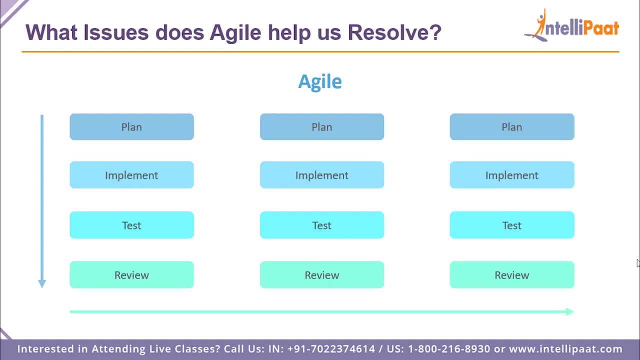 And similarly, you would go ahead and create the software as a whole. Now, in this manner, you're completing the software as well as providing the different components of software to the customer, getting her feedback and changing accordingly, Considering in all of 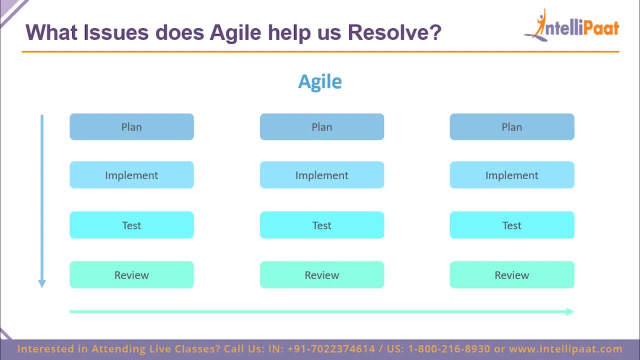 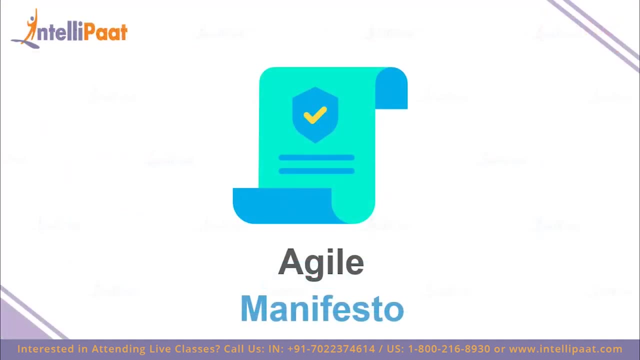 these factors, Agile's ability to change and adapt with the market, satisfy the market's needs and do so in a very short term. You know, all of these factors combined make Agile very suited for developing software these days. All right, guys. now I've called Agile a methodology, but in actuality it's rather a set of values. 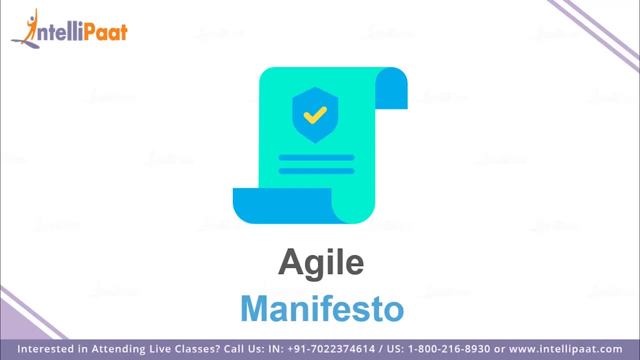 and principles. If you use these values and principles to make decision, then you're working in an agile manner. So, rather than being a methodology, it's rather a: basically, you set of values and principles that you have to follow if you want to be agile. Now let's. 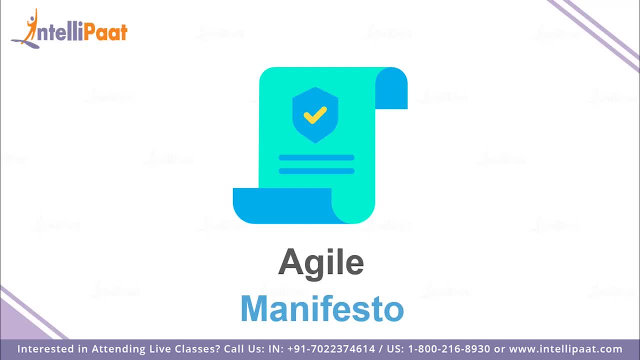 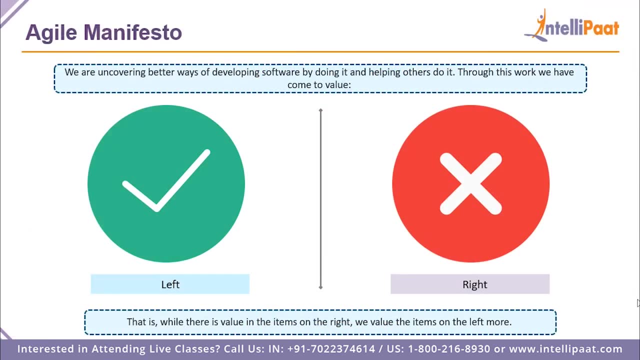 go ahead and discuss those values, those agile values. So they come under Agile Manifesto. So the Agile Manifesto basically states that we are uncovering better ways of developing software by doing it and helping others do it. Through this work, we have come to value. 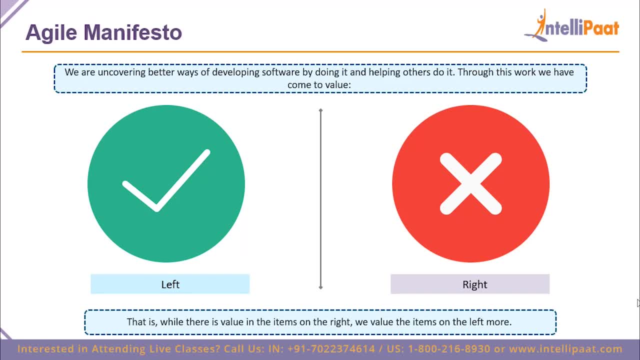 certain things. Now those. what are those certain things are the values. Now, what I'm going to do here is show you the left side compared to the right side, And this is how it's listed in the manifesto. also, You'll have a few values on the left. 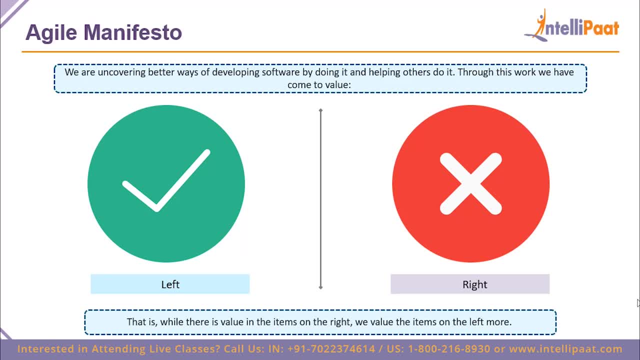 side and you'll have a value on the right side. While we have posted these values, we try to say that the left side values have much more meaning than the right side values. That is, while there is value in the items on the right also, we just value the items. 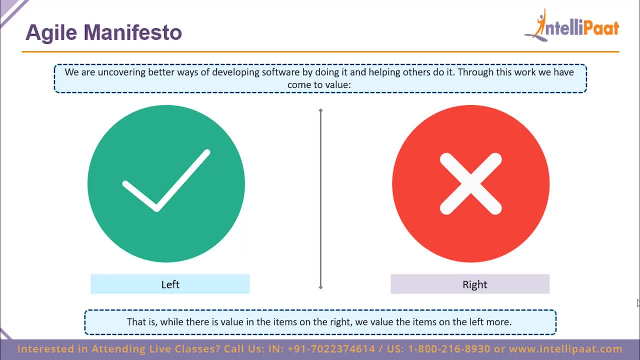 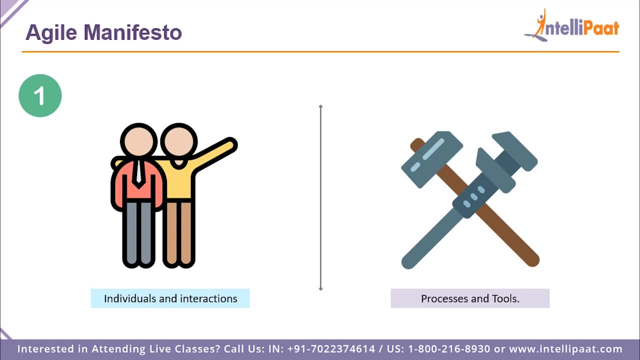 on the left more. Let me start off by giving you an example. So we have individuals and interactions and processes and tools. So individuals and interactions are on the left side and processes and tools are on the right side. So, even though we do value processes and tools, we just value individuals and the interactions. 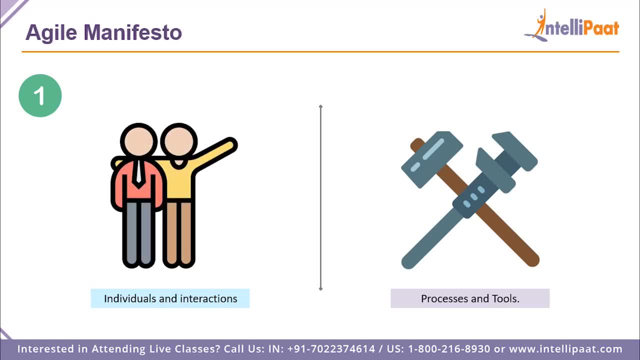 these individuals have between each other even more than the processes and tools involved, And this is the value that Agile promotes. This is the part of the Agile Manifesto. Now, there are similarly three more values, So let's discuss them also. We have working software. 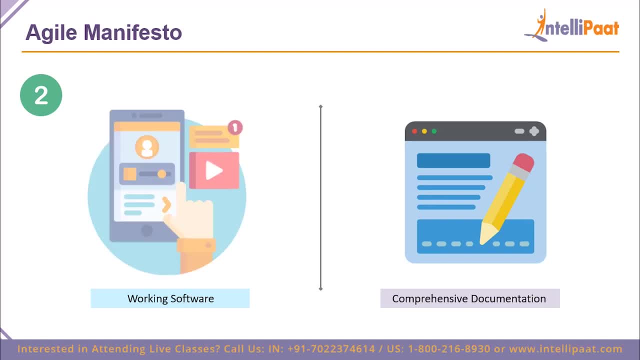 and comprehensive documentation. Here we value working software over having a comprehensive documentation, which is kind of obvious, right? So you have a functioning software that you're going to provide to your customer before you even have any type of documentation, Before you even think about going for documentation. 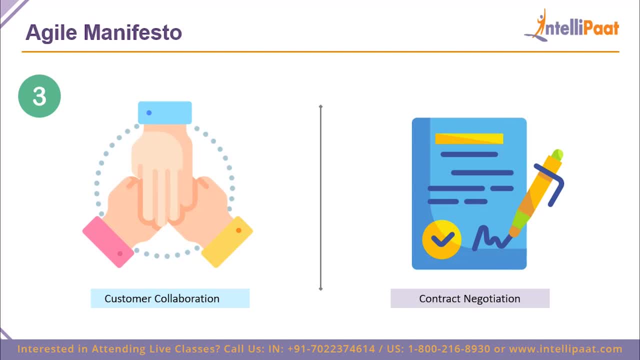 And this is what Agile promotes. And again, customer collaboration is valued more than contract negotiation, So we want to prioritize the feedback we get from customers and apply it into our software development over any type of contract that we're going to be signing with them. This is another value that Agile promotes And the final value that Agile promotes. 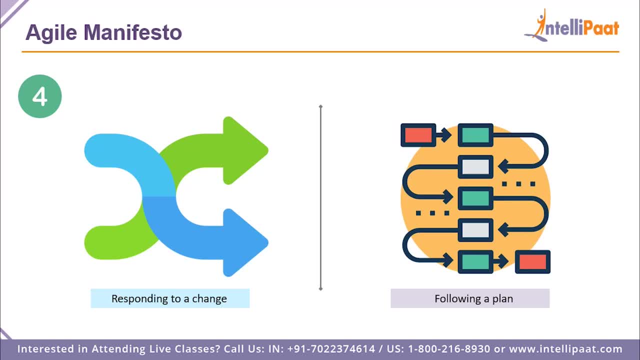 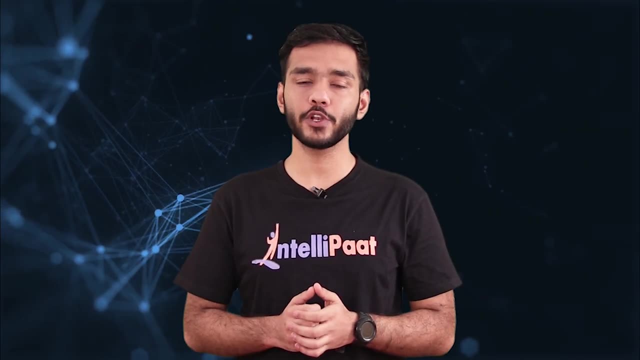 is basically responding to change. We value responding to change more than following a plan, because Agile is suited for, you know, ever changing market, And that's why responding to a change has greater value than following a plan. Quick info here, guys: if you're looking for end to end training in Agile, we do provide. 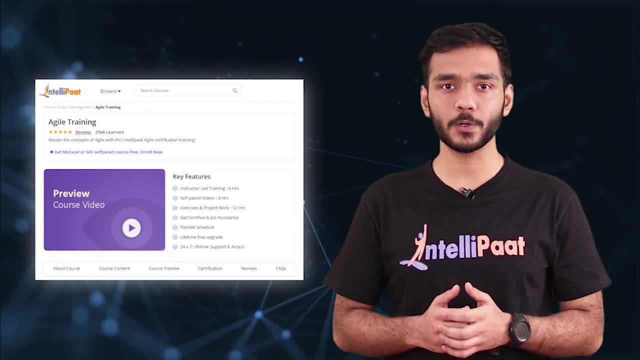 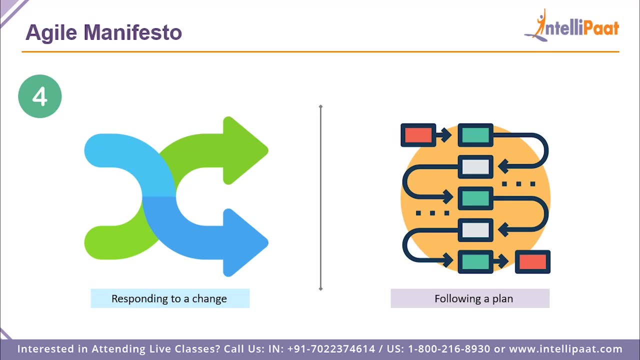 the same. For any further details, please check out the links given in the description below. And now let's continue with the session. So, guys, these are the different values that are promoted in Agile In the manifesto. if you ever read it by yourself, you will see that basically every item on 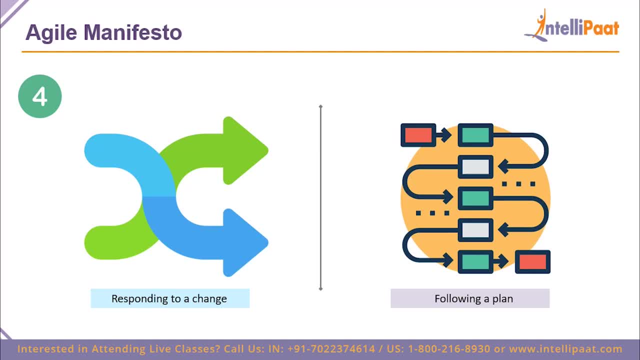 the left has more value than the item on the right. This does not mean that the items on the right are not valued. It's just that items on the left have just a lot more value, And that's why we have to follow them every time we are trying to make a decision. So whenever. 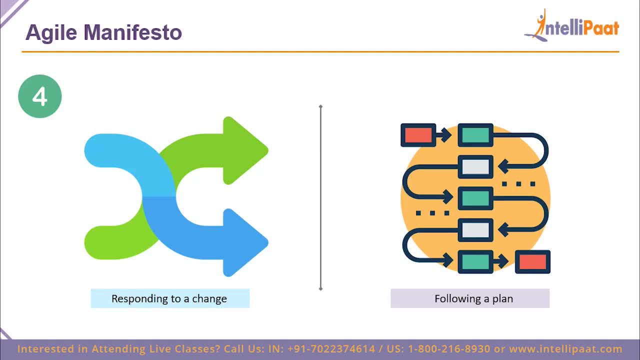 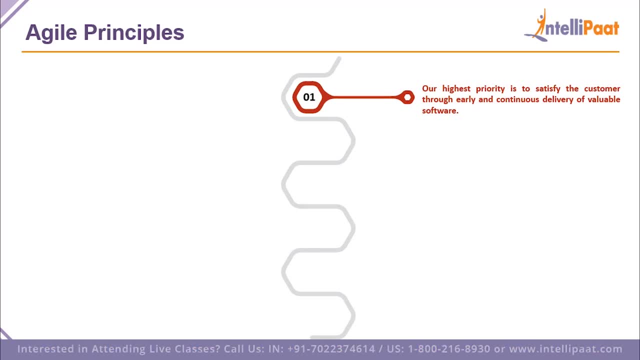 you make a decision, you have to keep these values in mind. Now let's discuss the different principles that Agile promotes. So we have the first principle that stays: that our highest priority is to satisfy the customer through early and continuous delivery of valuable software. The second principle states that welcome changing requirements. 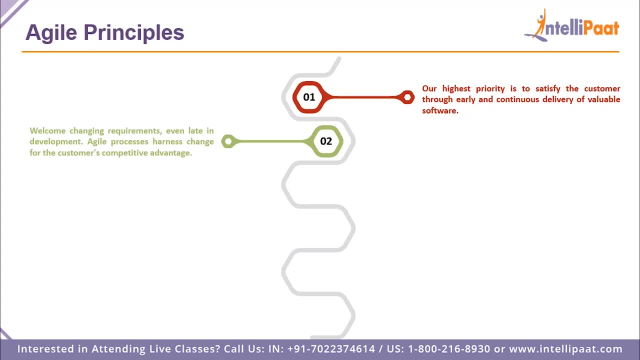 even late in development. Agile processes harness change for customers' competitive advantage. Then the third principle says that deliver working software frequently from a couple of weeks to a couple of months, with preference to shorter timescale. Then the fourth principle states that business people and developers need to be able to deliver. their products in a short period of time. This means that they need to be able to deliver their products in a short period of time. This means that they need to be able to deliver their products in a short period of time. This means that they need to be able to deliver. 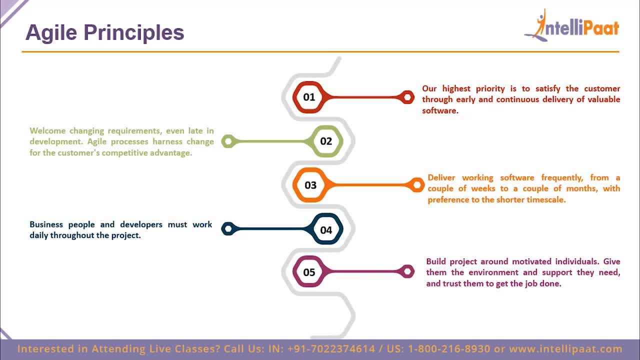 their products in a short period of time. The fifth principle states that we must work every day throughout the project. And the fifth principle states that build projects around motivated individuals, Give them the environment and support they need and trust them to get the job done. The next principle: 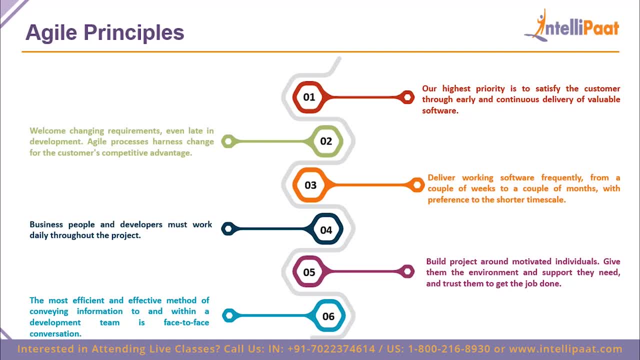 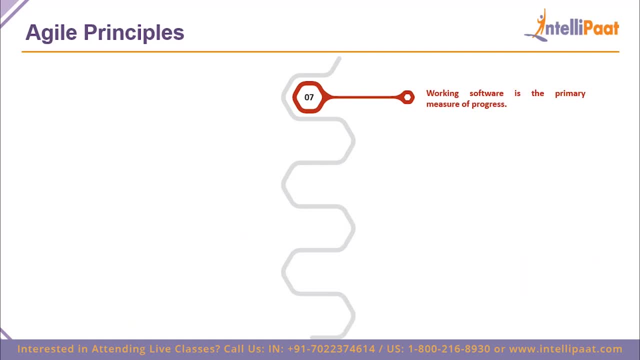 states that the most efficient and effective method of conveying information to and within the development team is face to face conversation. The next principle states that working software is the primary measure of progress. Then agile processes promote sustainable development. The sponsors, developers and users should be able to maintain a constant pace indefinitely. 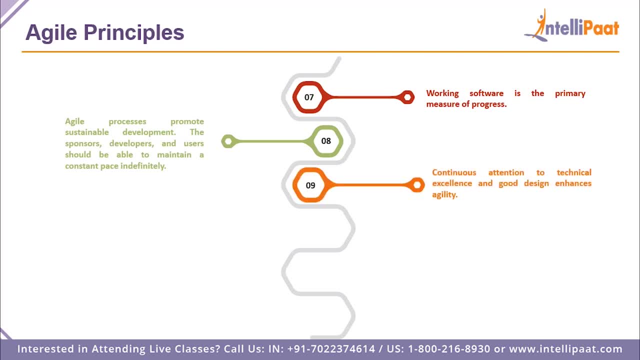 The ninth principle states that continuous attention to technical excellence and good design enhances agility. Then simplicity, the art of maximizing the amount of work not done, is essential. And the second last principle states that the best architectures, requirements and designs emerge from self-organizing teams. 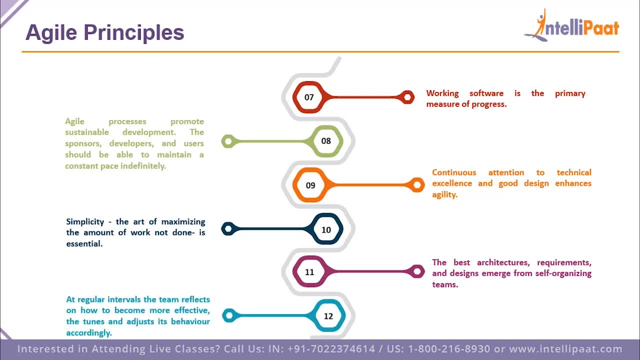 And the final principle basically tells us that, at regular intervals, the team reflects on how to become more effective, then tunes and adjusts its behavior accordingly. So, guys, these were the different principles that agile promotes. Now remember, if you want to be an agile team, then you have to make all of your decisions. 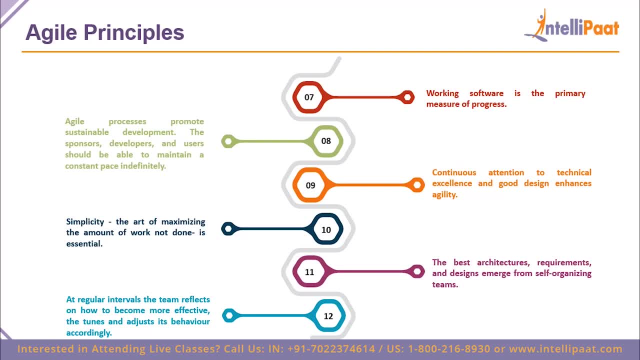 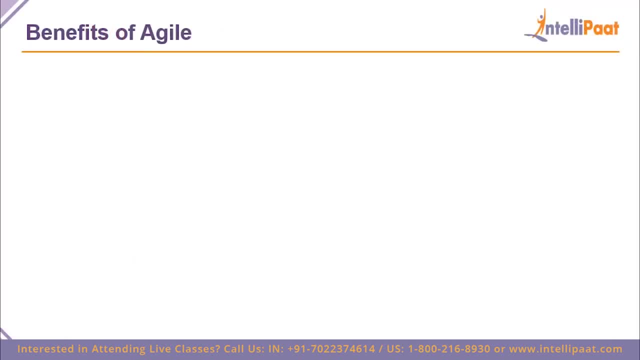 based on these principles and based on the values that agile promotes. Otherwise, you are not an agile team. All right, now let's look at the different benefits that agile provides us. So the first benefit is basically transparency. Now, this is pretty clear by the idea of transparency itself. 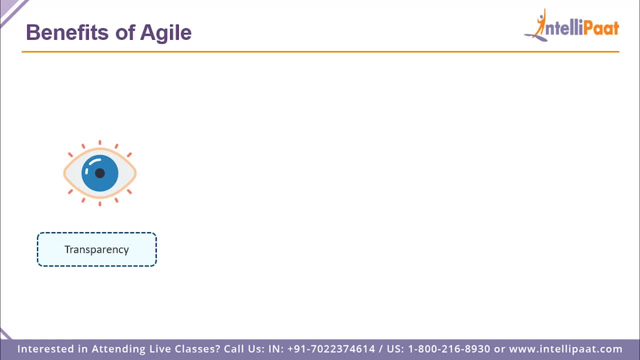 If you are transparent in your development process, then the customer or the client knows what you're doing. They have more trust in you because you'll be telling them what you're doing, and you'll be doing this as you'll be providing them software every other sprint. they'll know. 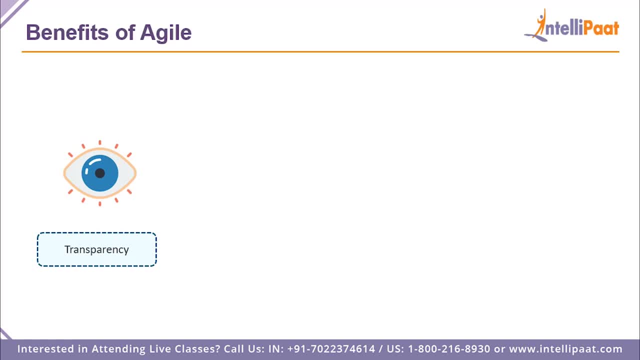 what kind of software they're getting and accordingly they'll provide you a feedback and you will improve upon the next iteration by using that feedback in your planning stage. Then comes predictable costs and schedule. Now, since agile promotes very short term development life cycles, the number of variables that 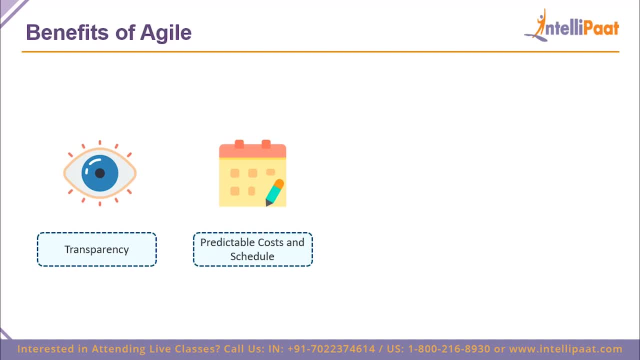 will be there when you're calculating the costs and schedule will be less, and hence you'll able to predict the cost and schedule all the tasks much more efficiently. Now, another benefit- and it's a primary benefit- is that it allows for change. Now, the values and principles that agile tells us about basically promote for change, because 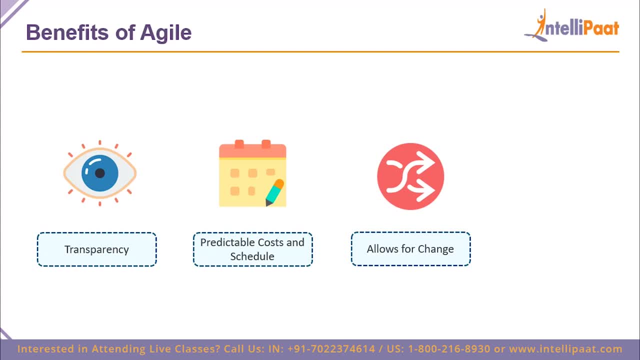 if you are able to adapt and change according to the market. Okay, If you are able to increase your business profits as well as satiate the market's needs or as well as satisfy your customer or client, and then in the end, it helps us to improve. 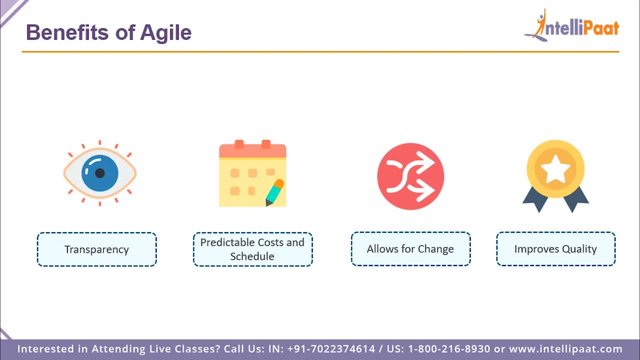 the quality of the product overall, not just the polishing aspect. you increase the morale of your employees, you increase the morale of your team, and this way they want to make a better product and hence a better product is made. So these are the benefits of agile. 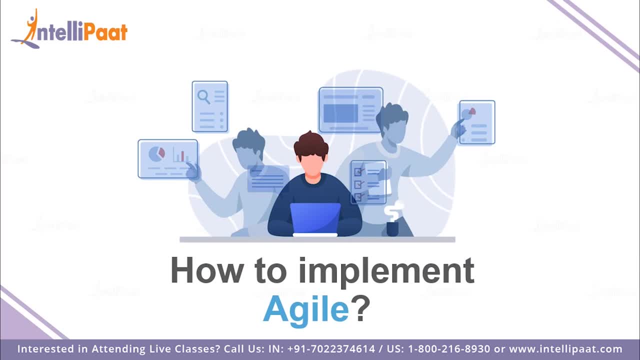 Now let's move on and see how we can implement agile ourselves. Now, whenever you're going ahead with implementation, Implementing agile, you have to keep in mind that any decision you take has to be based on the values and principles set by agile. 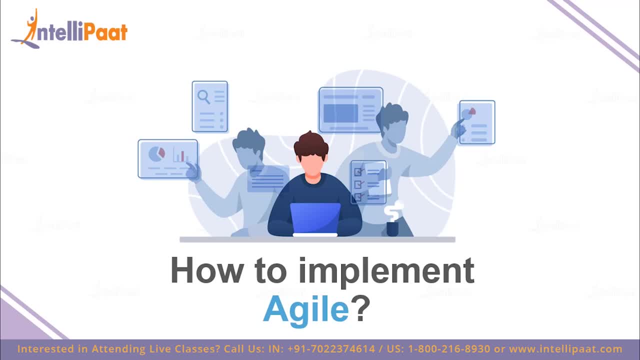 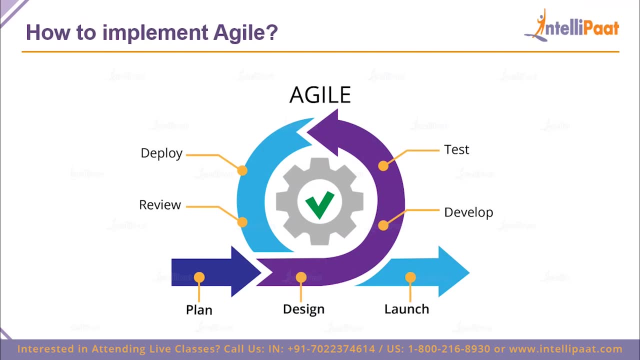 Otherwise, you're not going to be having an agile development, All right. So when you're going ahead with these principles and value set in your mind, you have to follow the normal sprints. Now they're going to be a lot of practices that you'll have to choose from. 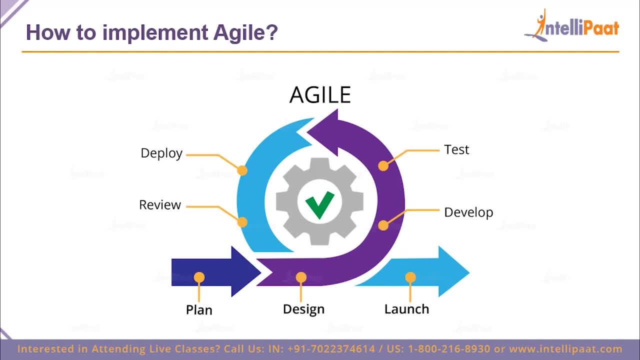 Now one of the practices is to having a sprint, where you have a small sprint, small iteration, where you develop a small component of the software And give it to the client. So you'll first plan it out, then design it, then develop it, then test it, then deploy. 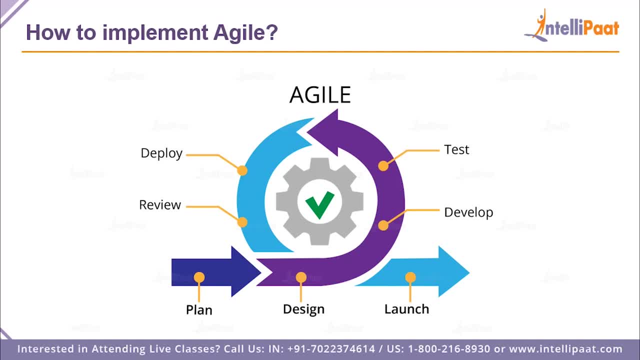 it, then review it from your own feedback, from the customer's feedback, from the client's feedback, then launch it and you know, then move on to the next iteration. Now this is a part of the practice of agile, So there are a lot of agile practices out there. 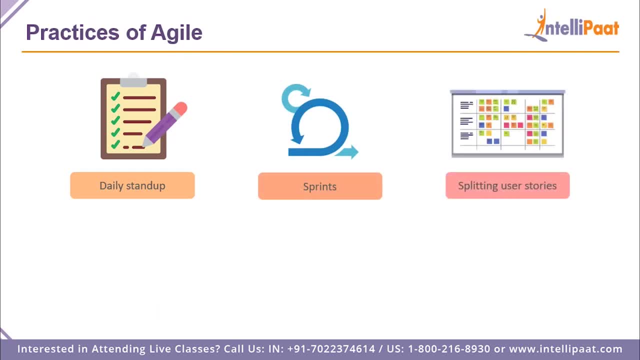 You have a daily standup, sprints, splitting user stories, pair programming and test driven development. Now you can go ahead and choose any practice you want to, But remember, You have to choose these practices based on your own needs and based on the values and 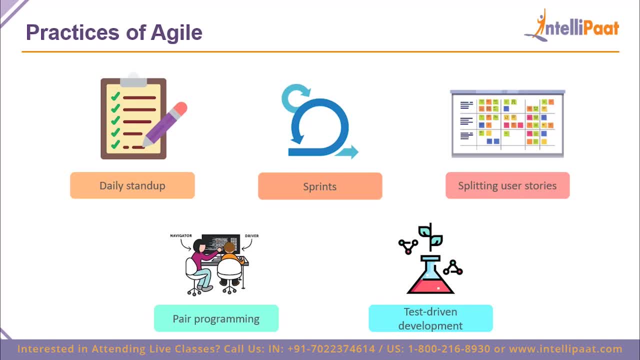 principles that are being set by agile or that have been promoted by agile. Otherwise, you're not agile or you're not following an agile development, And hence you won't get the benefits of agile. So keep this in mind when you're going ahead with any of the practices of agile. 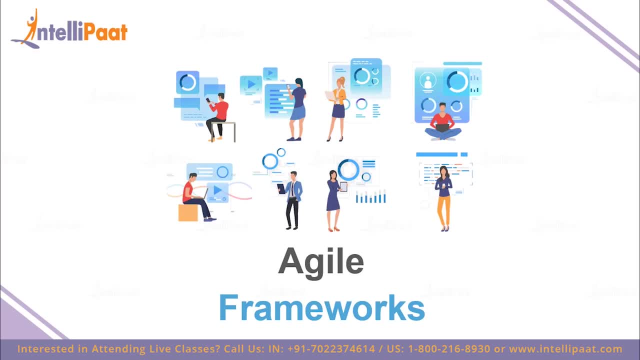 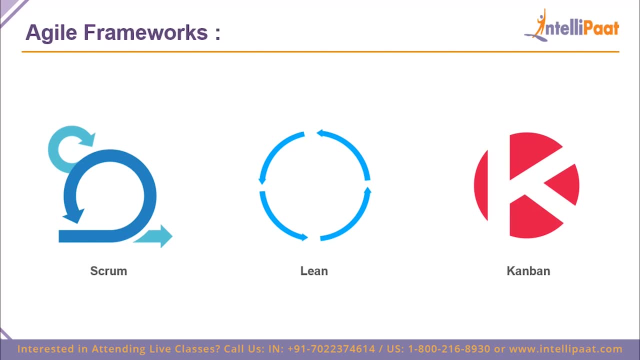 All right, Now let's move on and discuss the different frameworks of agile. So with Scrum, you're focusing more on the openness, the focus, the commitment, the courage and the respect for different people, Whereas in lean, you're trying to focus on eliminating all the waste, amplifying as much.